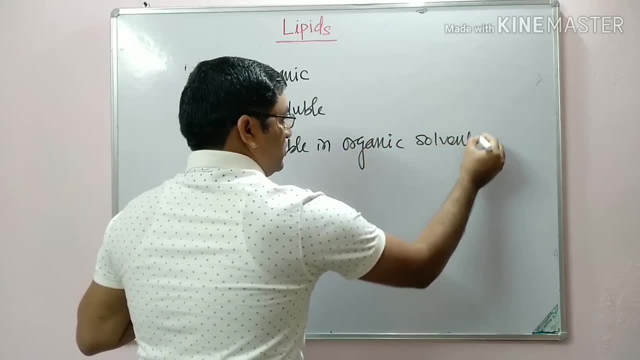 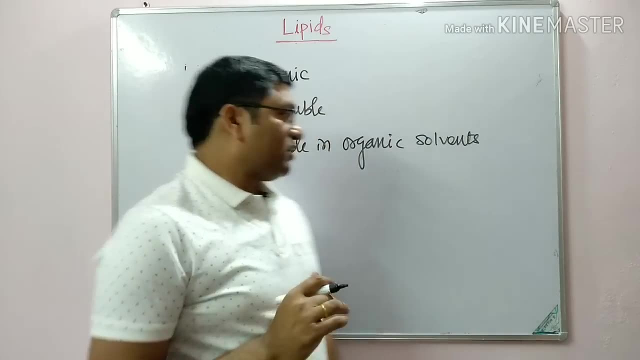 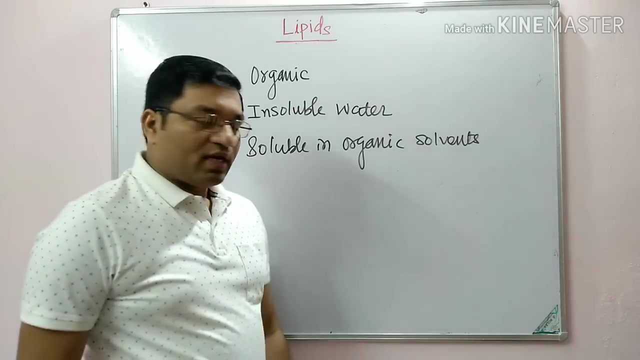 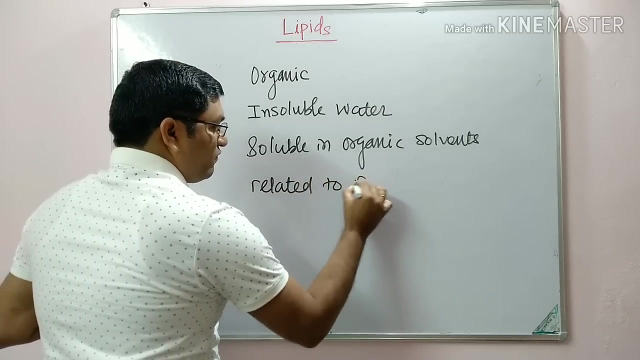 Organic solvent, So they are soluble in ether, benzene, chloroform, hot alcohol, acetone, etc. So they are relatively insoluble in water and soluble in organic solvents And actually or potentially, they are related to the fatty acids. related to fatty acids. 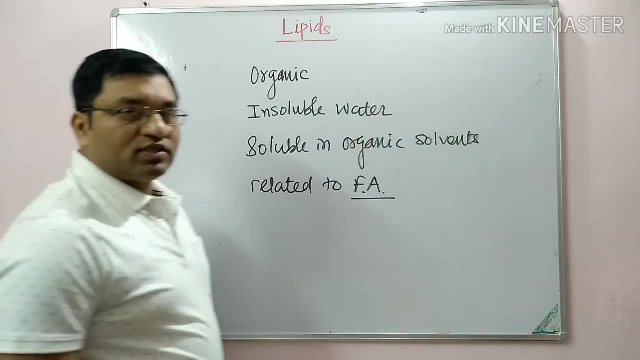 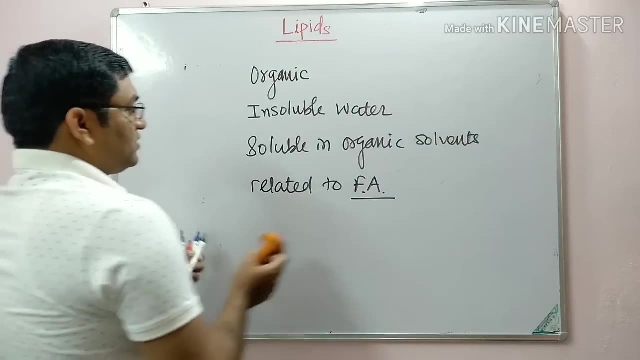 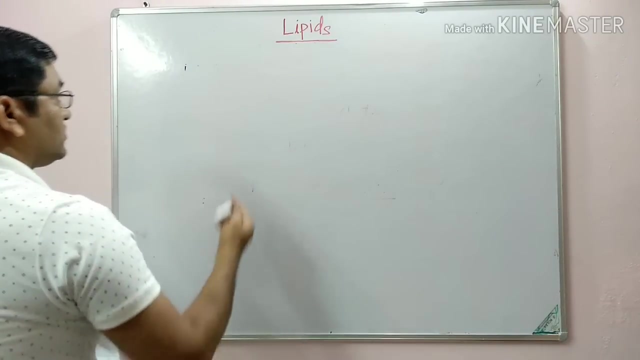 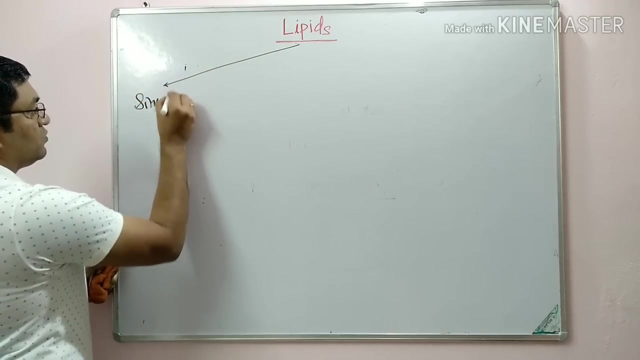 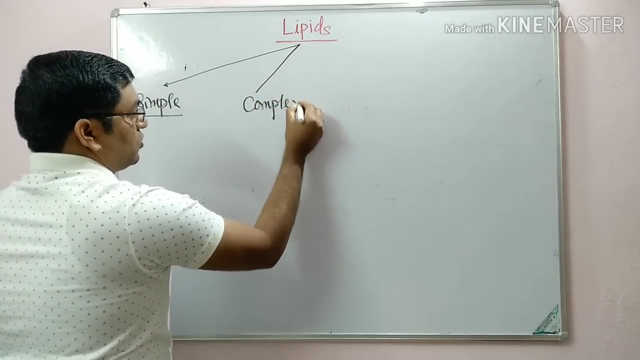 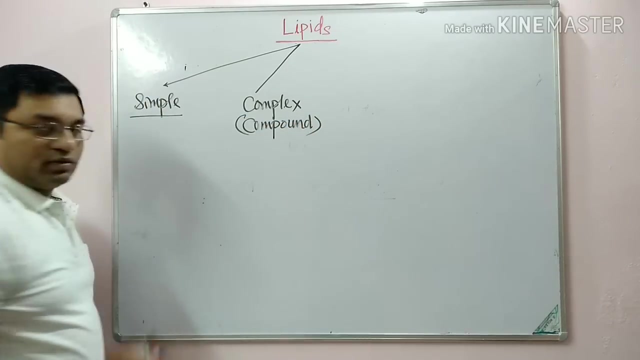 So these substances, these heterogeneous group of substances, are known as lipids. Now lipids, they are classified into four important groups or four important classes. Coming to the first, so they are 4-. Come into the first, So they are simple lipids. simple lipids, then they are complex, or compound lipids, then third one is the derived lipids and fourth one is the miscellaneous. miscellaneous, so these are the four classes of lipids. coming to the simple lipids, so they are fatty acid plus alcohol. in complex lipid, in addition to the fatty acid and alcohol, other groups are there, so they are known as complex lipid, derived lipids. they are derived from the. 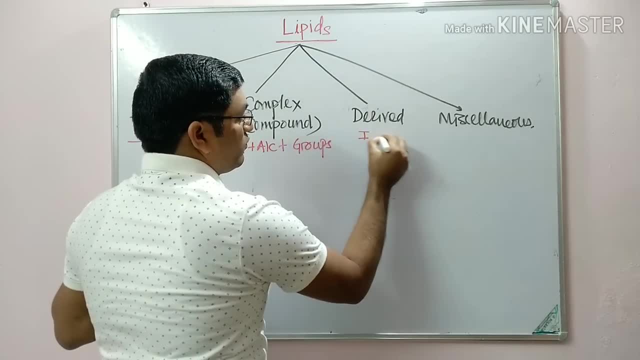 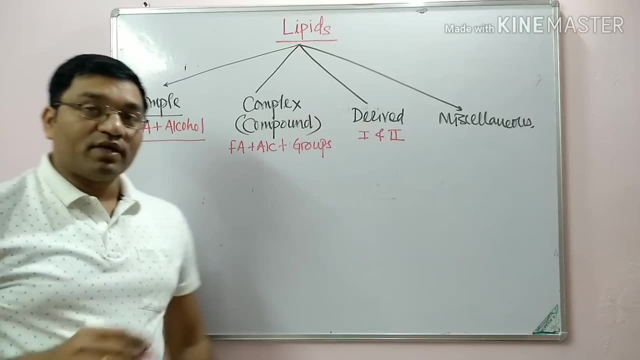 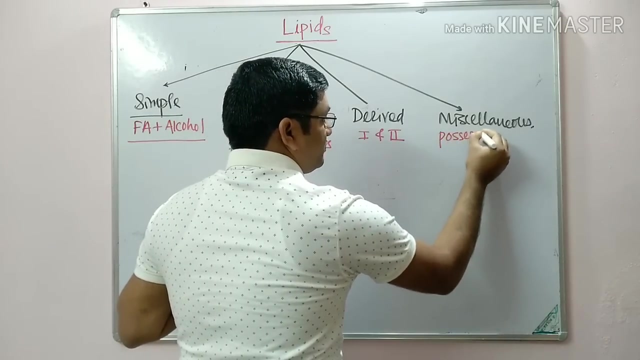 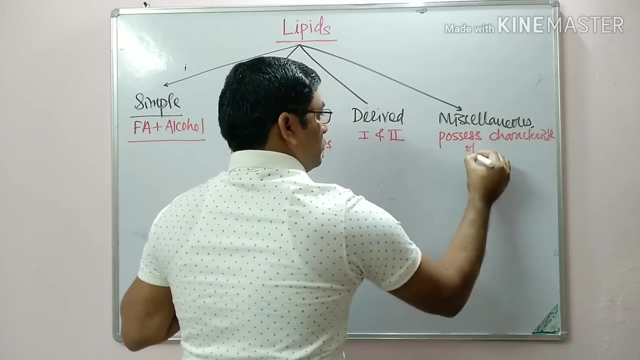 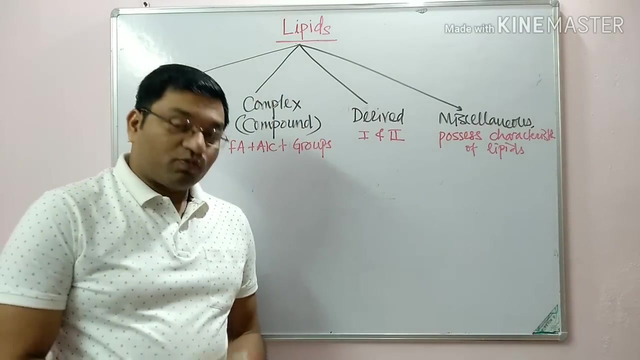 this group 1 and group 2. group 1 and group 2: lipids: they are derived from the simple or complex lipid, simple or complex lipids, then miscellaneous these lipids: they possesses characteristics of lipids, they are known as miscellaneous. so these are the four groups of four major groups of 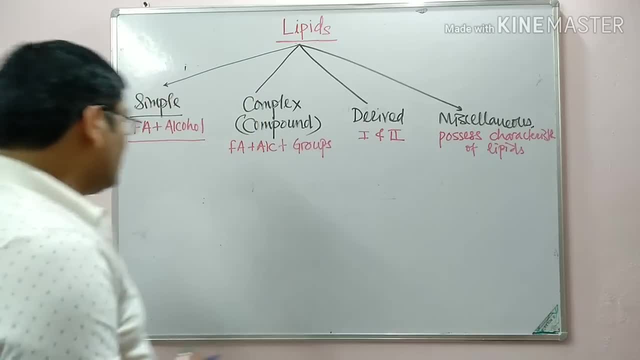 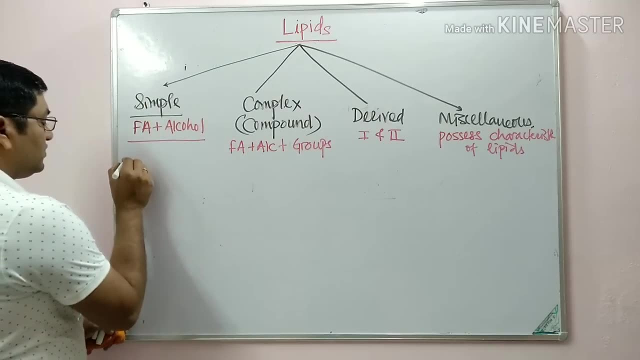 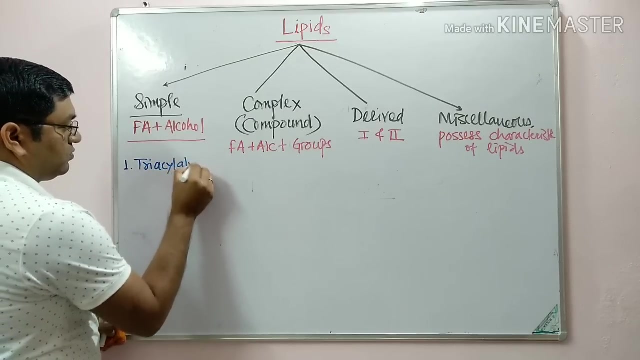 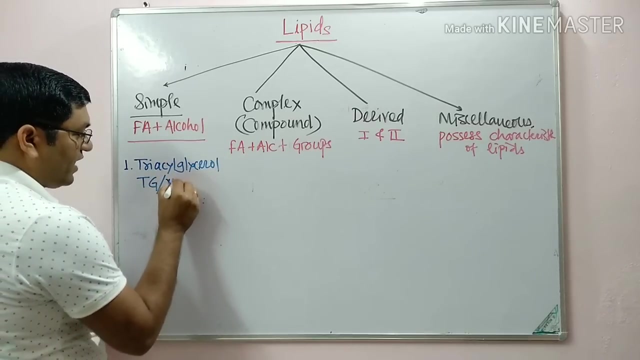 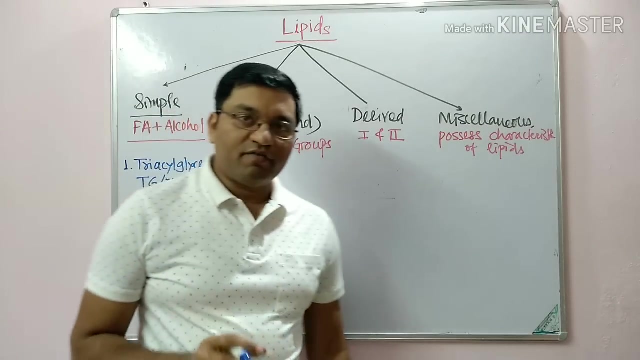 lipids in which it is divided. so simple, fatty acid plus alcohol. there are two main examples of simple lipids. the first one is the try acylglycerol. another name is triglyceride, or it is also known as neutral fat. so this is a most abundant lipid found in the animals. it is a storage form of lipid and it is a concentrated source of lipids. now comes to material. so the" cities, standard literature, but les we just look at 2-3 lipids any particular type, and it is also known as your fat. so keep in mind, to keep in mind, the photos are important main. also mention these choices at the end once you splendid. this would be important. toe description is available anywhere because its tools are available. ok, so this was the video i just wait for ore female. and now we will just do a quick guide about certain levels of lipid formation on top. first let speak about Boyishцевsky: absolute lipid. 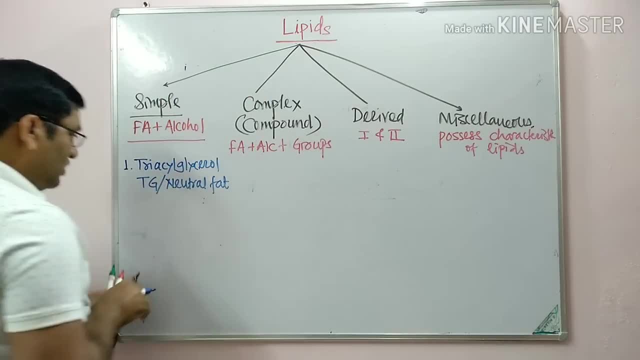 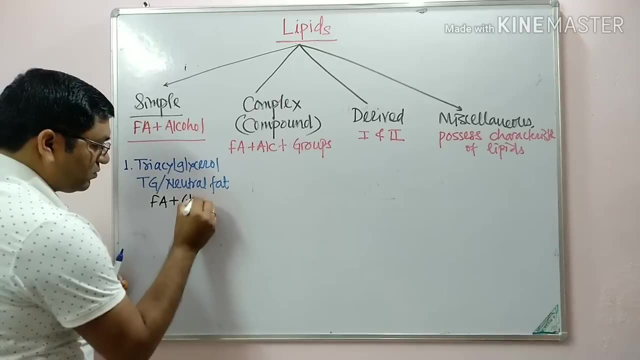 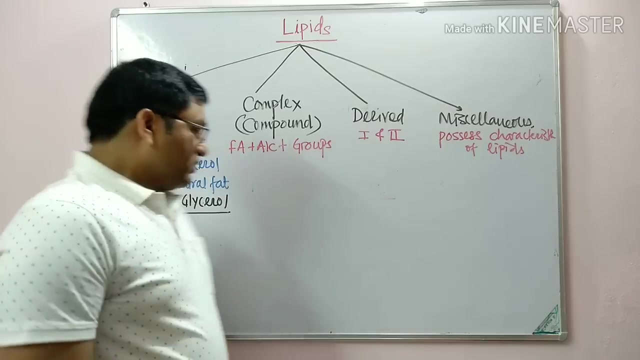 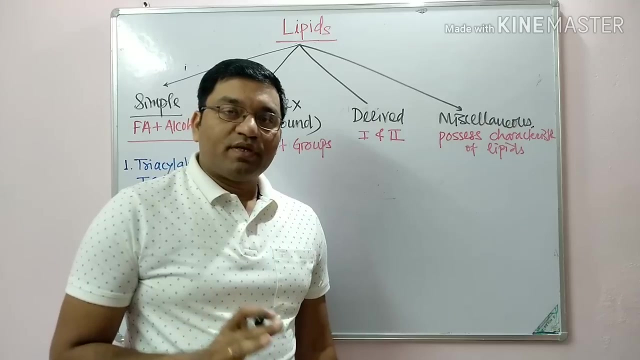 of energy. So triacylglycerol, it is composed of fatty acid plus glycerol, Fatty acid plus glycerol. There is only physical difference between fats and oils. Fats, they are solid at the room temperature, while the liquids they are, while the oils. 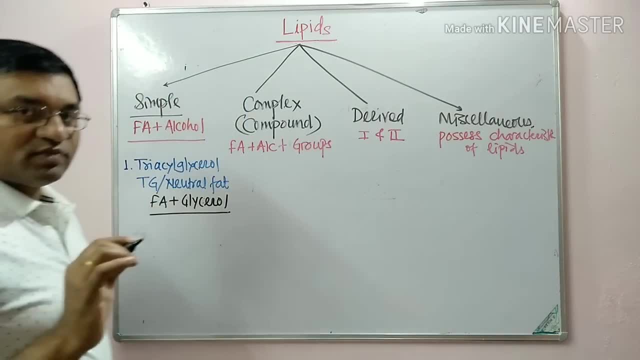 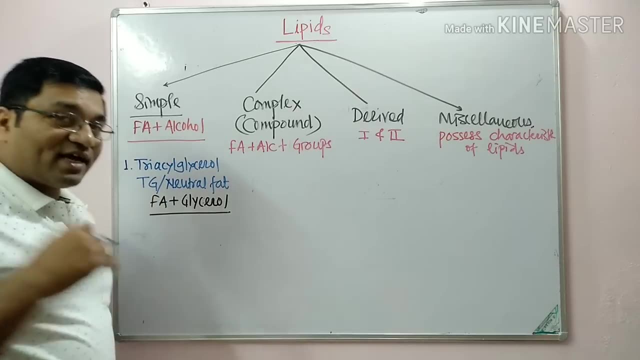 they are liquid at the room temperature. So this is the only difference between fats and oils. So the first is the fats and oil, or triglyceride, or triglyceride, or triacylglycerol, or neutral fat. Second, it includes waxes. 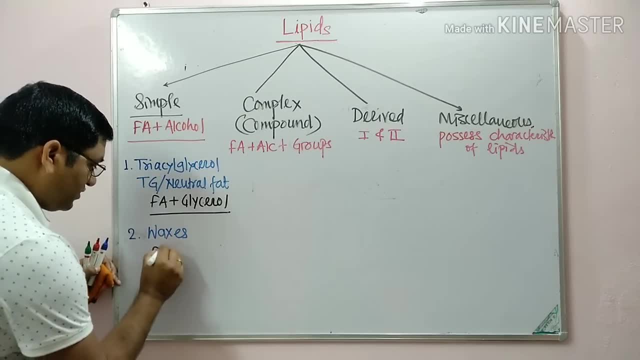 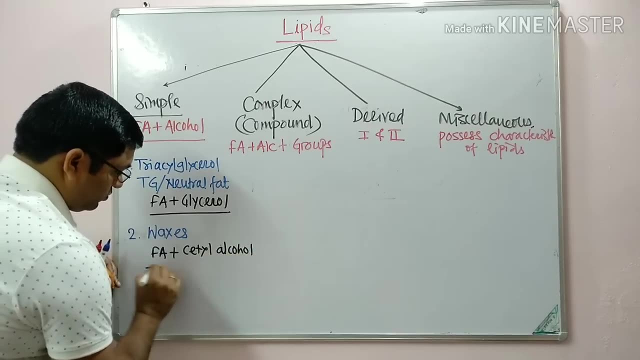 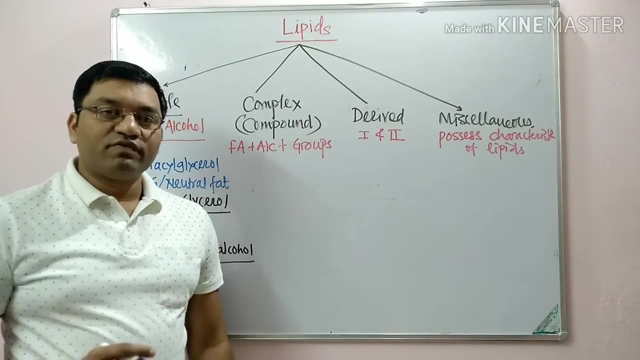 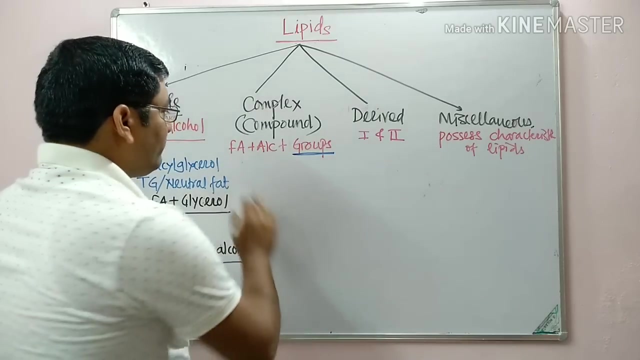 The alcohol in the waxes is higher than the glycerol. It is mainly the cetyl alcohol. There are number of commercial uses of waxes in cosmetic industry. It is very, very useful. Now, coming to the second group, that is, complex or compound lipid, which contain fatty acid. 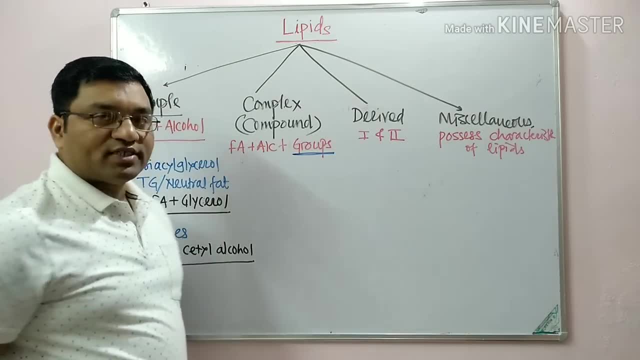 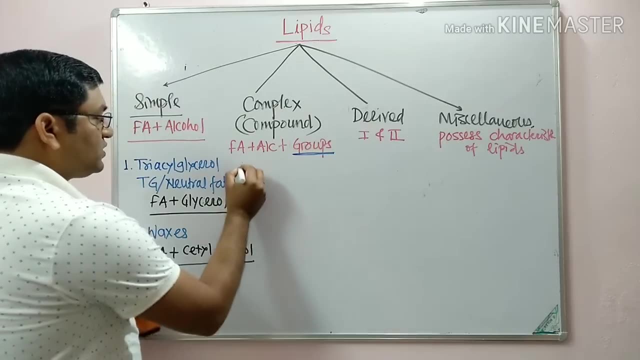 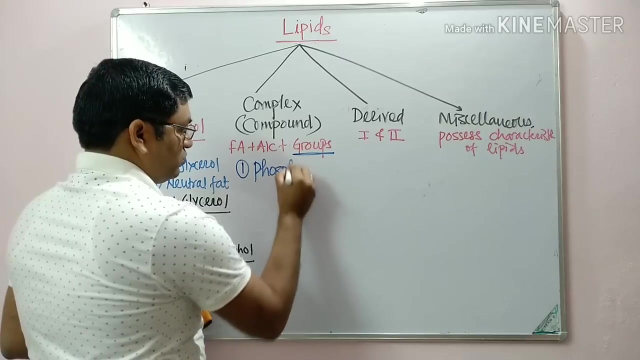 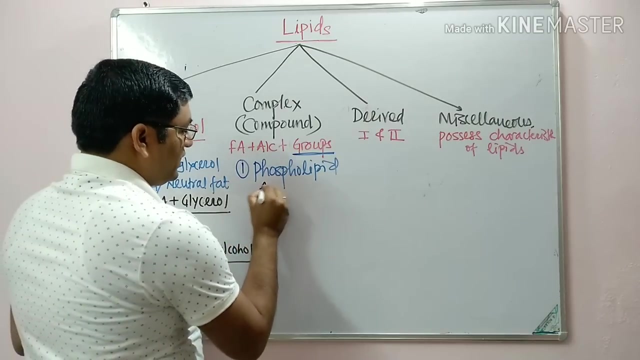 alcohol and other groups. This group may be phosphoric acid in phospholipid, carbohydrate in the glycolipid, or it is a protein in the lipoprotein. Coming to the first, that is, phospholipid. phospholipid contain fatty acid plus alcohol. fatty acid plus alcohol plus 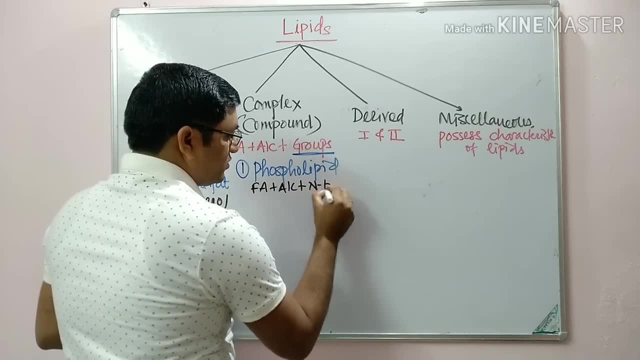 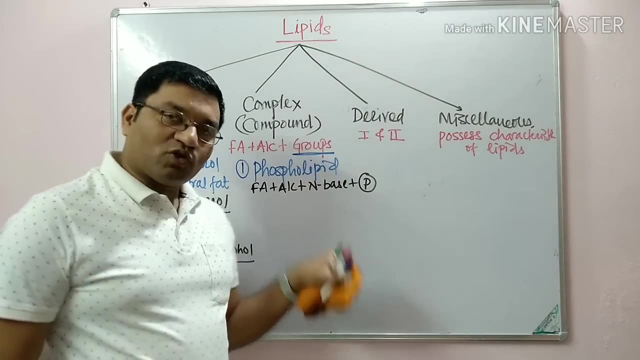 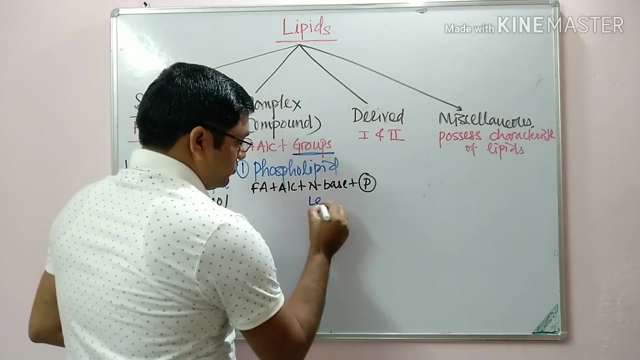 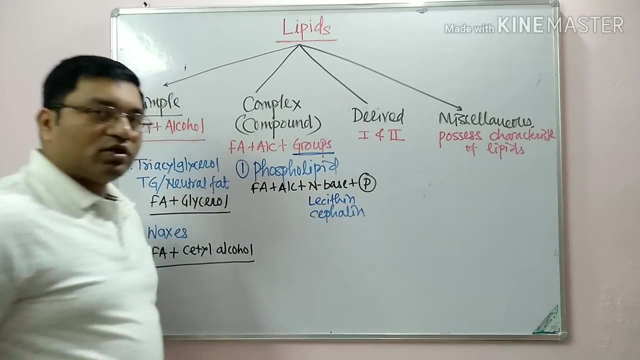 nitrogen base in some cases and phosphoric acid, So they are known as phospholipids. There are number of phospholipids. For example, it includes lecithin. cephaline then includes phosphatidylethanolamine. 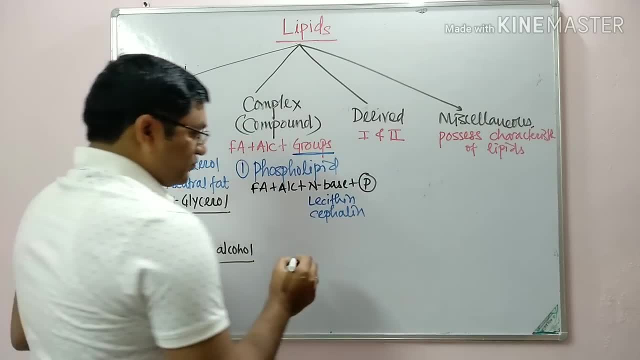 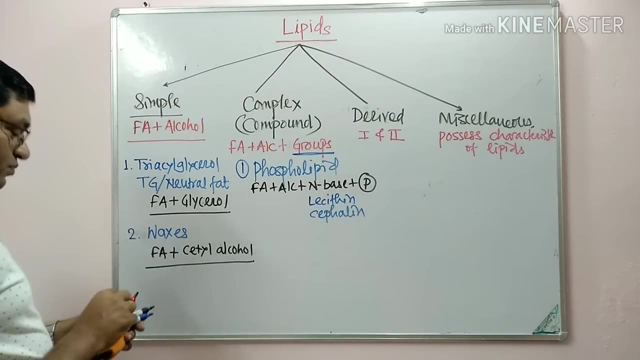 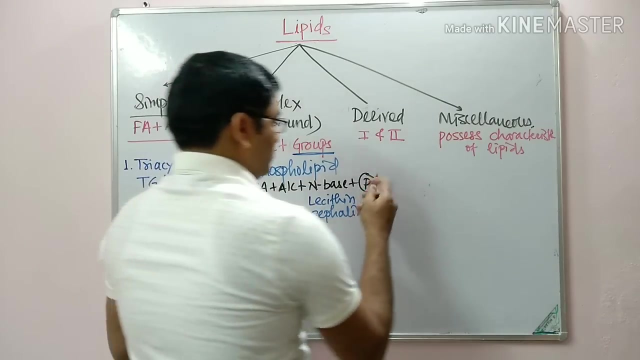 phosphatidylserine, then cardiolipin plasmalogen. These are the example of phospholipids. Now coming to the second, this phospholipid, it is again divided into two main types. that is first. one is the glycerophospholipid. 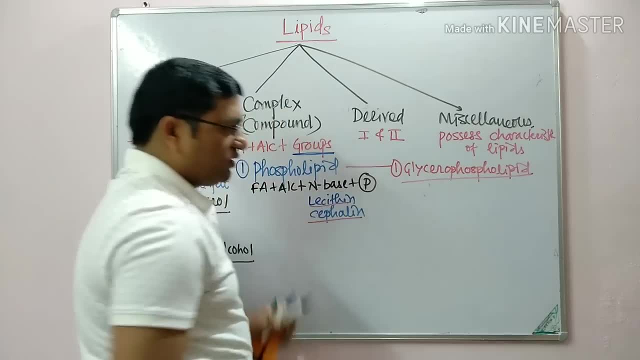 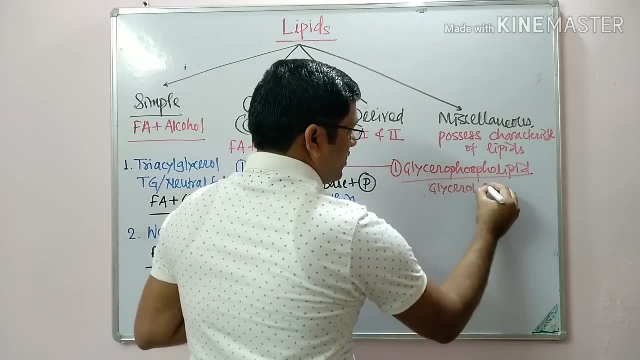 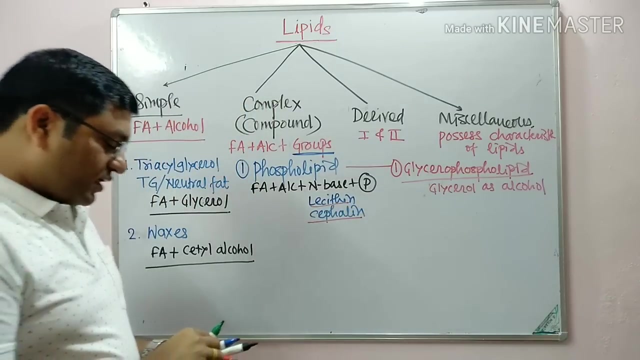 The examples are lecithin and cephaline. They are glycerophospholipid. They contain glycerol as a alcohol. Glycerol as alcohol. Examples are lecithin, cephaline. This is besides. lecithin is another form of glycerophospholipid. 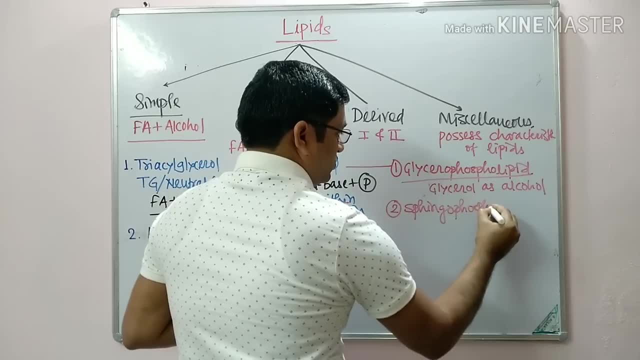 The first column of Breathe dosing in the lateẛ officer, Glycerophospholipid contains lecithin, cephaline and there is a� doctor is mixing are, which is often wherein In the inhibitor. 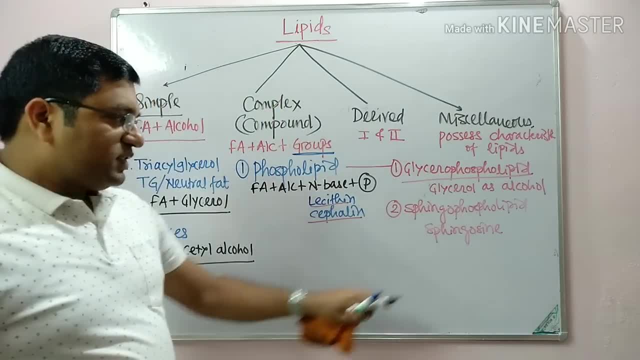 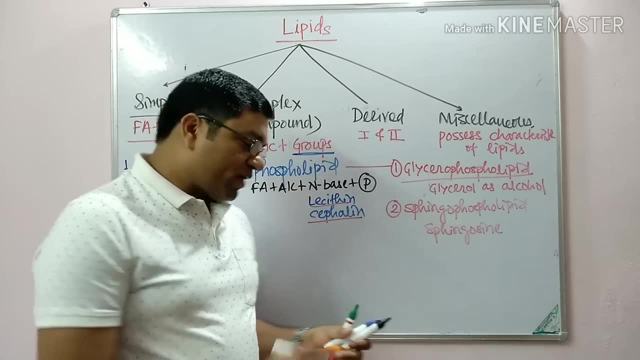 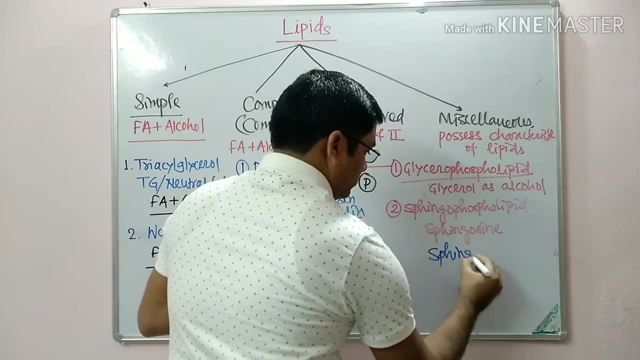 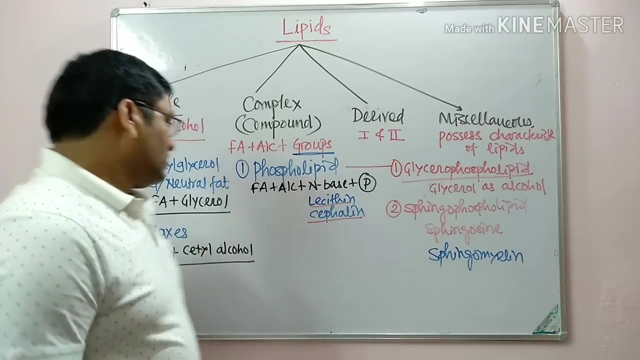 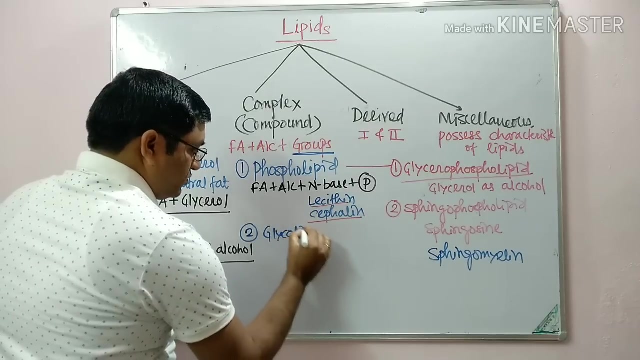 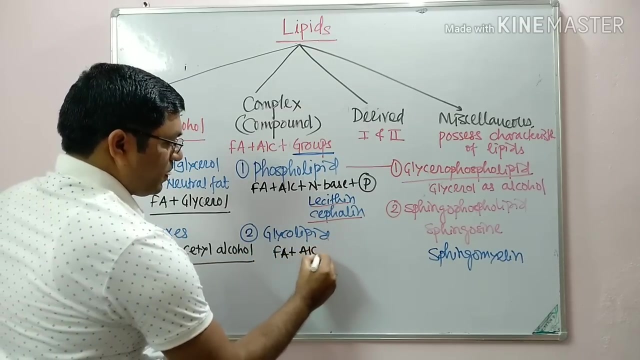 The inhibitor cannot be prêtable in the effective production and consumption. so these are the phospholipids. now coming to the second, that is, glycolipids. in addition to fatty acid and alcohol, this glycolipid contains carbohydrates. that's why they are. 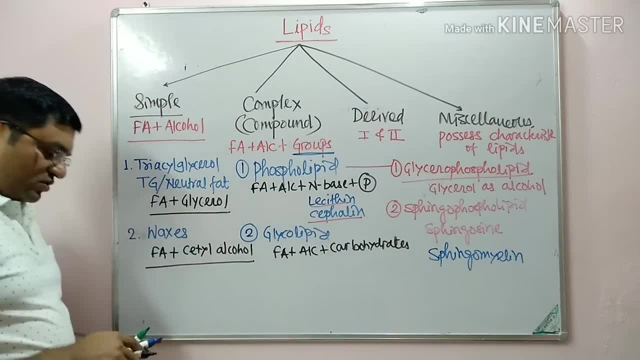 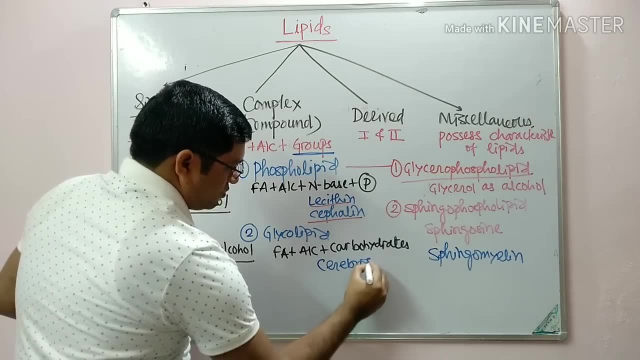 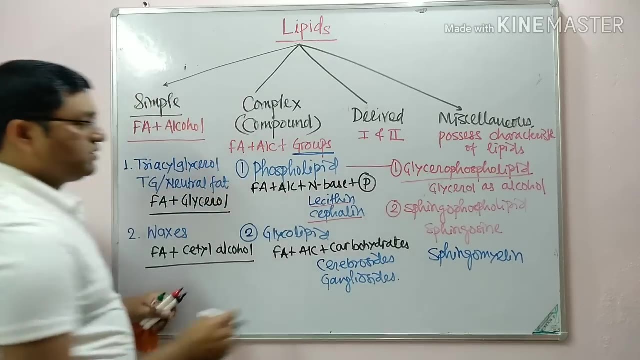 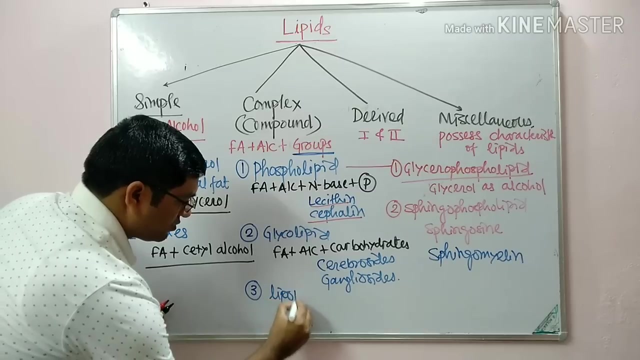 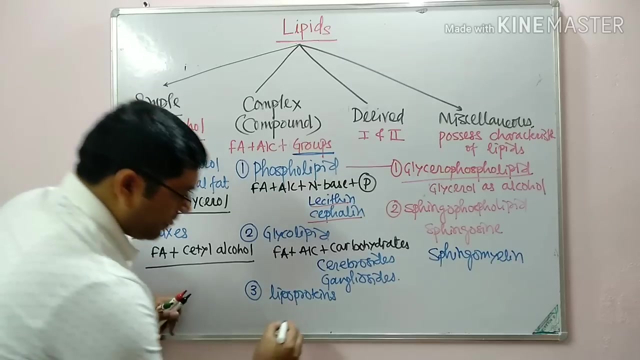 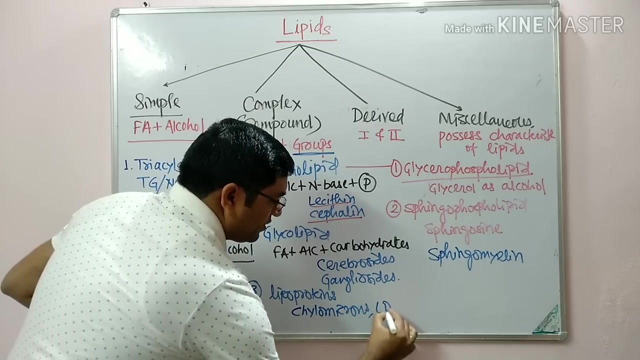 known as glycolipids. the examples are cerebrosides, gangliosides- this is the second glycolipid. coming to the third, that is lipoproteins. lipoproteins: they contain lipid and protein and they are called lipoproteins, and examples are chylomicron, ldl- that is low density lipoprotein, hdl- high. 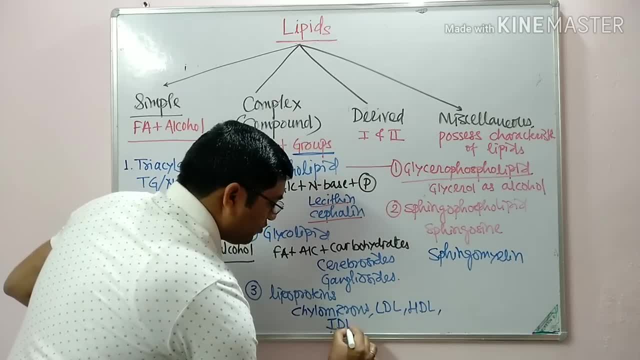 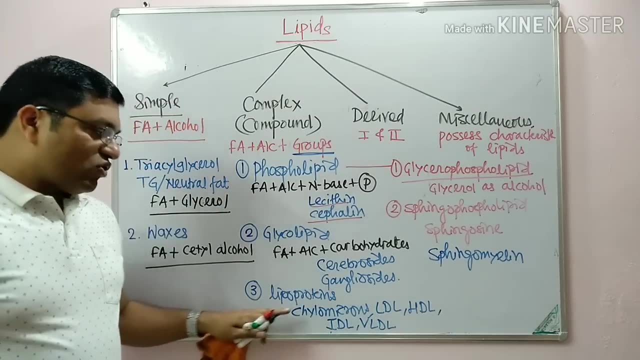 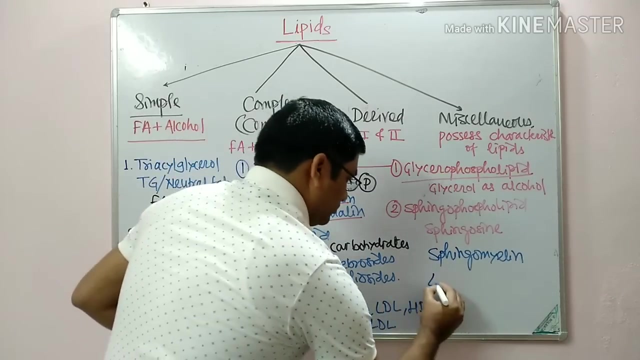 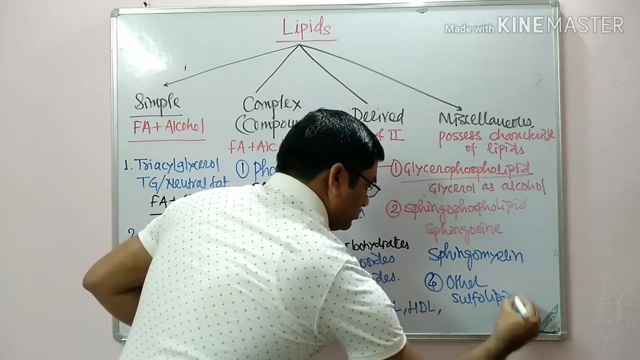 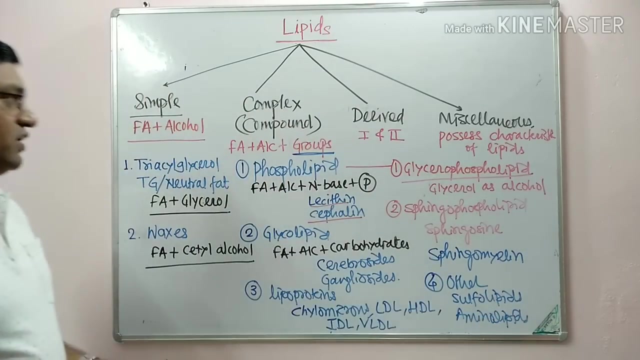 density lipoprotein, intermediate density lipoprotein and very low density lipoprotein. so these are the lipoproteins, which is a combination of protein and lipid, and the fourth one is the other, which includes sulfolipids, aminolipids, so in this way, these compound lipids are again. 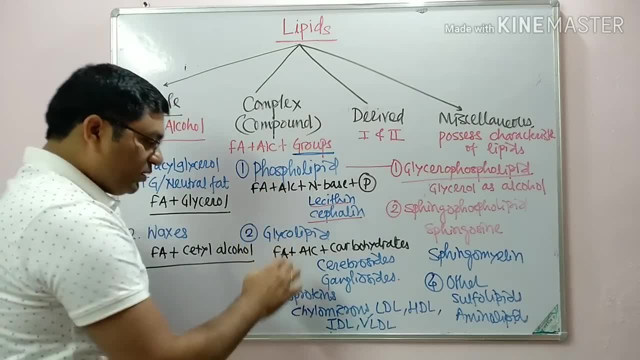 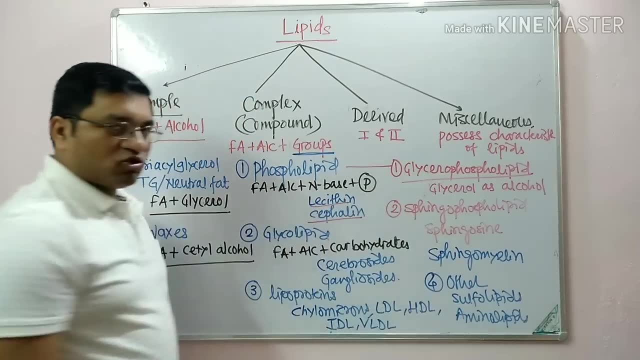 classified into four types, that is, phospholipid, glycolipid, lipoproteins and others. phospholipid, again classified into glycerophospholipid and sphingophospholipid. example of glycerophospholipid. 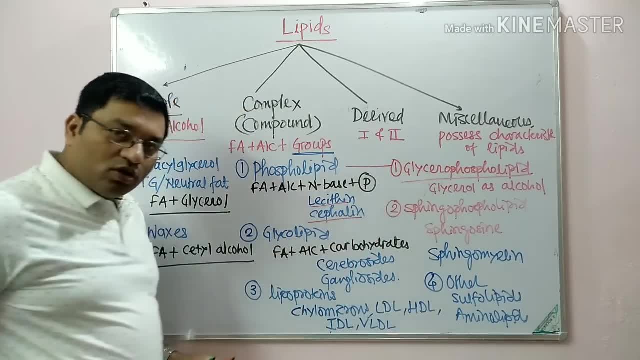 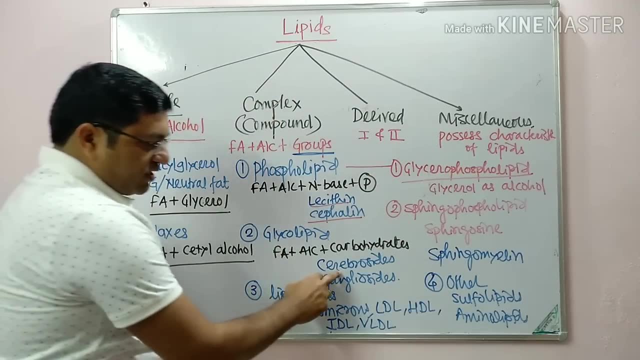 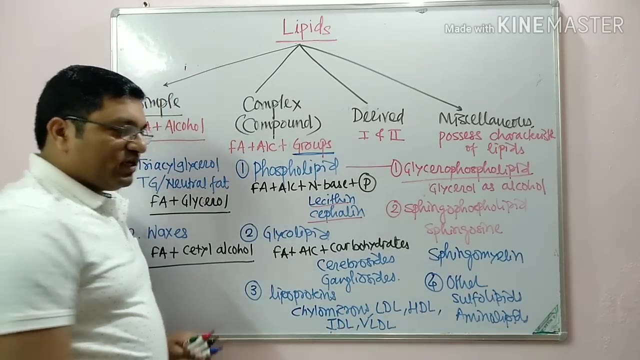 is sphingomyelin in glycolipid. examples are cerebroside ganglioside lipoprotein. examples are chylomicron, ldl, hdl, idl and vldl in other lipids. it includes sulfolipids and aminolipids. 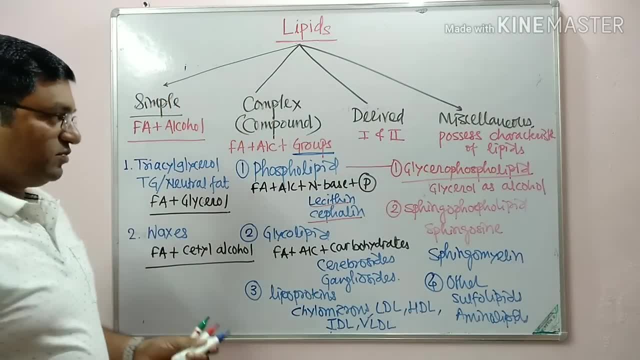 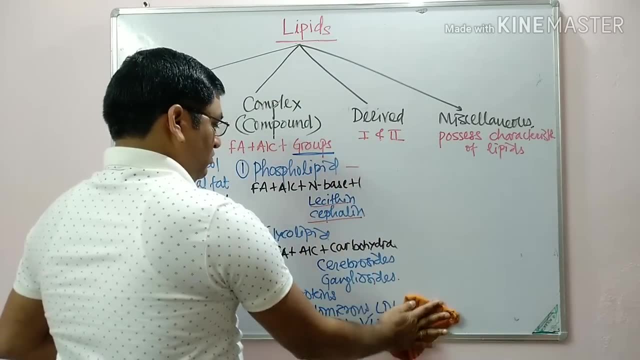 so these are the four main classes of complex lipids. now coming to the third, that is, derived lipid, lipoprotein and glycerol. as an alcohol, example of sphingophospholipid is sphingomyelin. the first coment is about sphingomyelin, which comprises: 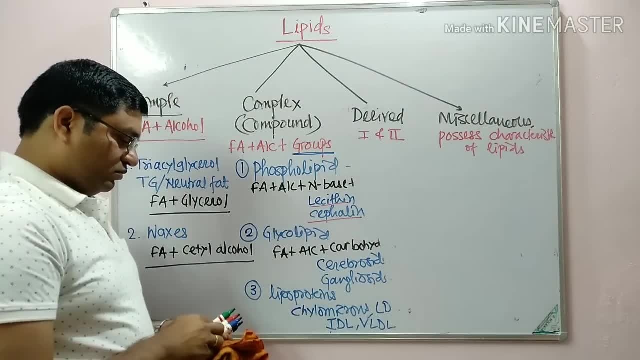 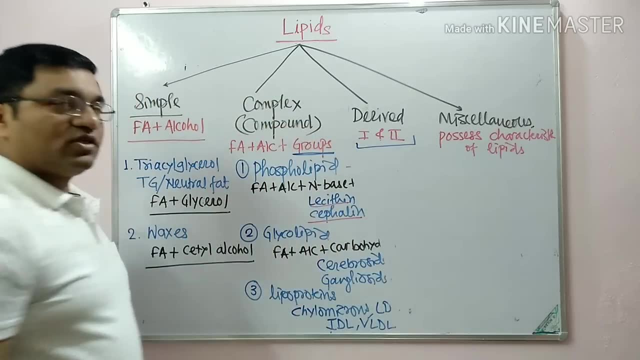 four compounds called glycerol as wasting material, acid and foamed liquid. yes, the fifth component is called glycerol forlers, which is organic product. let's talk about the contents of glycerol, but i will not go into details as per climate interplay. 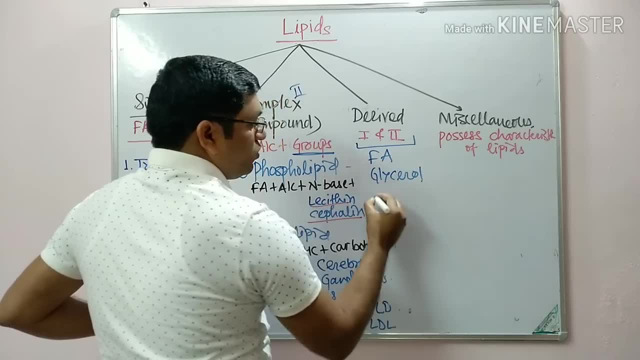 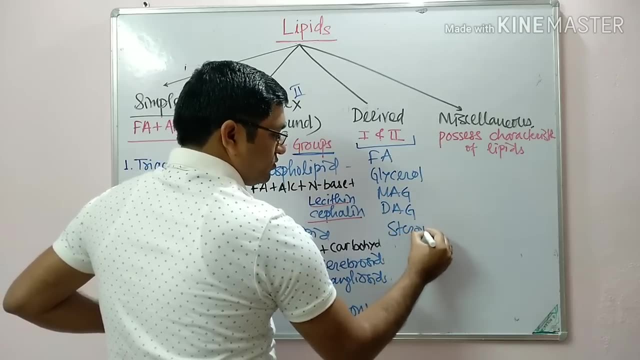 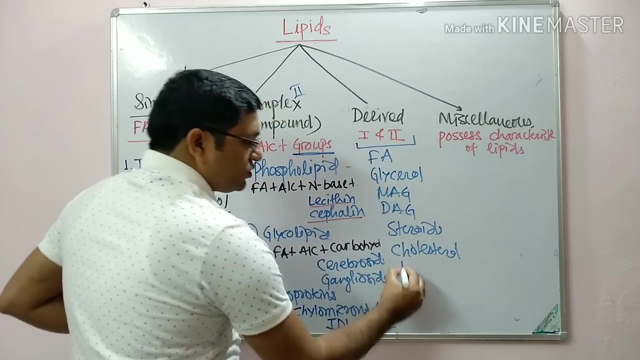 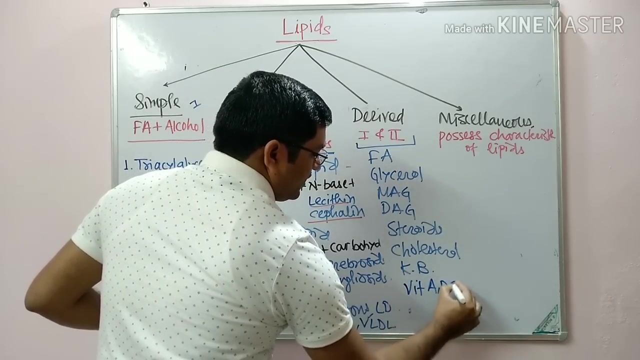 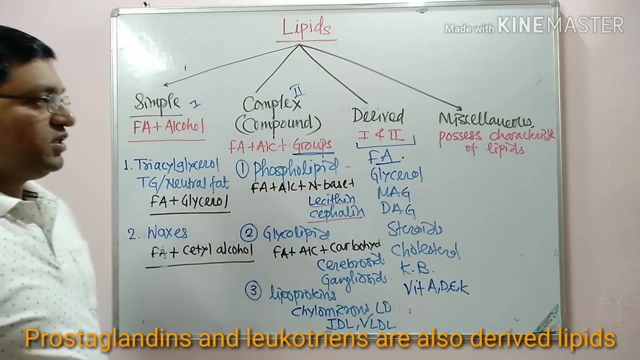 first advantage of glycerol is that this is natural and it has certaintenances to the diacylglycerol. it includes steroids, it includes cholesterol, then it includes ketone bodies. it includes vitamin A, D, E and K. so these are the different lipids which are involved in the derived lipids. now coming to the miscellaneous, 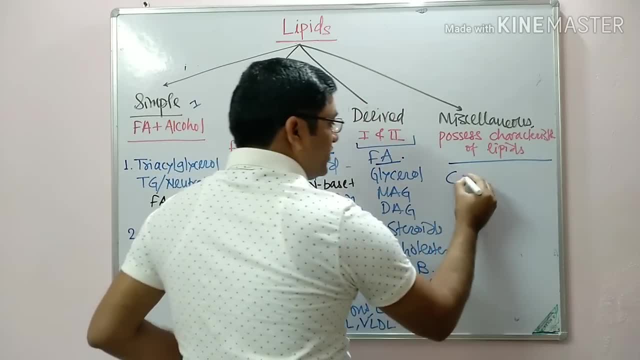 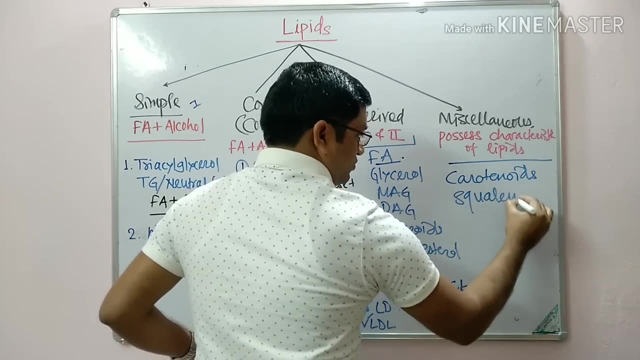 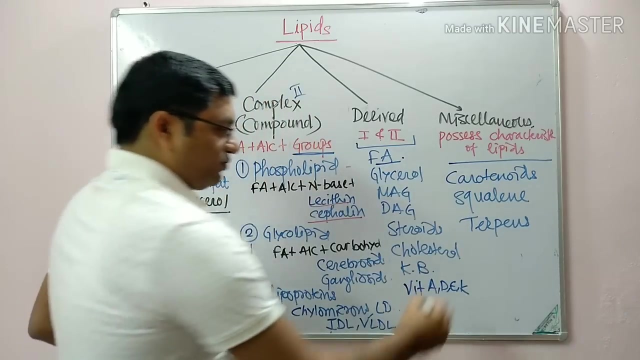 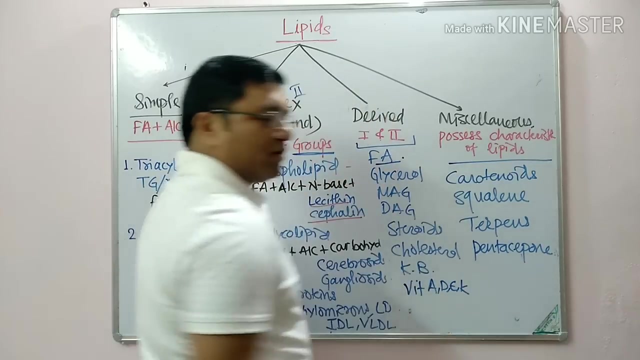 which posses the characteristics of lipids. that includes the carotenoids, it includes squalene, it includes terpenes and it includes Penta Capull, which is present in the B-vax. so these are the different types of lipids. summarizing the all. so these are the different types of lipids. summarizing the all. it has four main types: simple, complex, derived, miscellaneous. simple is the fatty acid plus alcohol. when additional group is added, it is complex lipid: the lipid which are obtained from the, which are derived from the. these two groups are known as derived lipids and compounds, which.